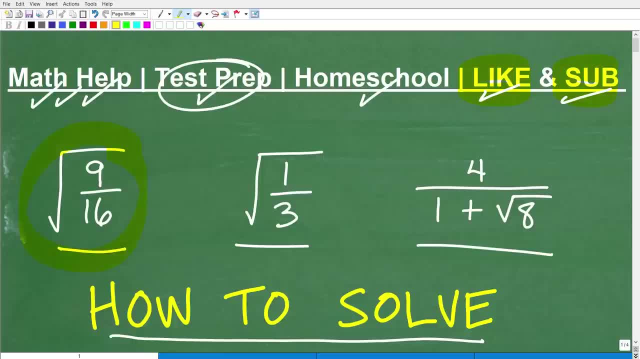 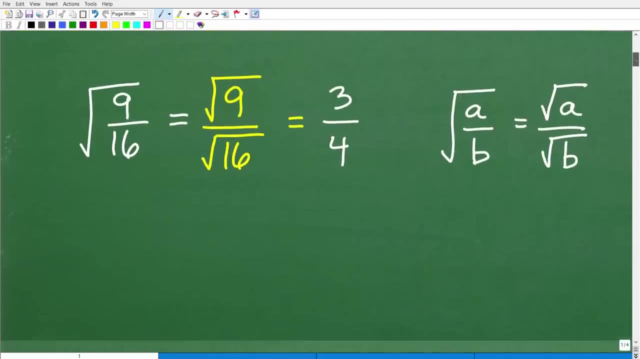 All right, I'm going to kind of lay this out here. We're going to do this problem first- This is going to be the easiest- And then we're going to go on to this problem. This problem has a bit of a twist, And then this one here is much more involved. So let's get to it right now and talk about this first problem. 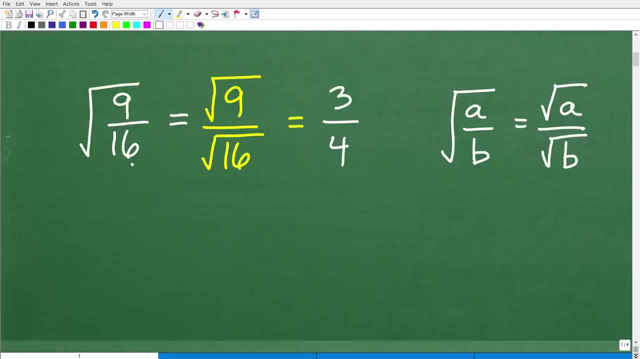 All right. so how do we find the square root of 9 16ths? Well, we need to know this property right here, You can see I already wrote out the answer, But here's the main idea. If you're taking the square root of a fraction, okay, and you have one big square root of A over B, well, that's equal. 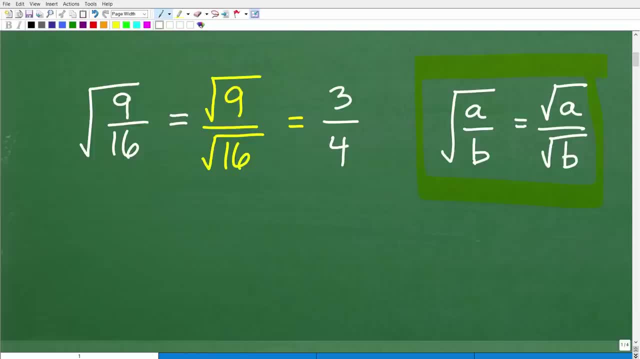 To taking the square root of the numerator over the square root of the denominator. So you can kind of break this up. You can either take the square root of the entire fraction or you can have two little square roots, one for the numerator and one for the denominator. 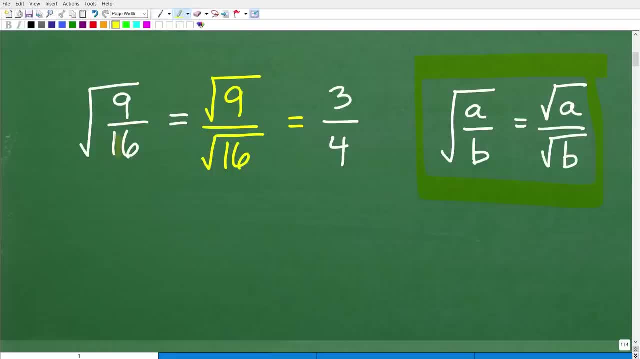 So you can kind of see it this way. So the square root of 9 16ths this fraction. I can write this as the square root of 9 over the square root of 16.. And then, of course, I can easily find the square root of 9.. 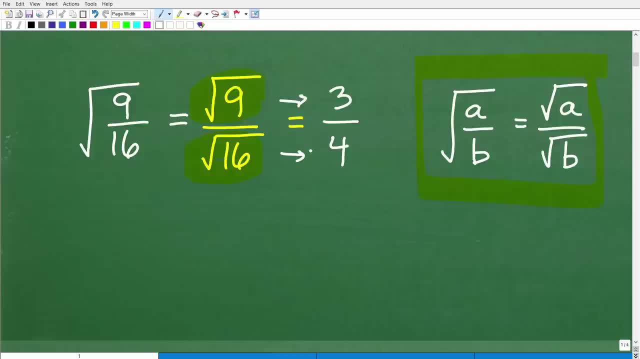 That is 3 and the square. Now let me mention something here to you real quick. When we're discussing basic square root problems, things like this, you want to just stick with the principal square root. In other words, here the square root of 9 is equal to 3.. Although some of you might be thinking, oh, isn't the square root of 9 equal to plus or minus 3?? That is true. 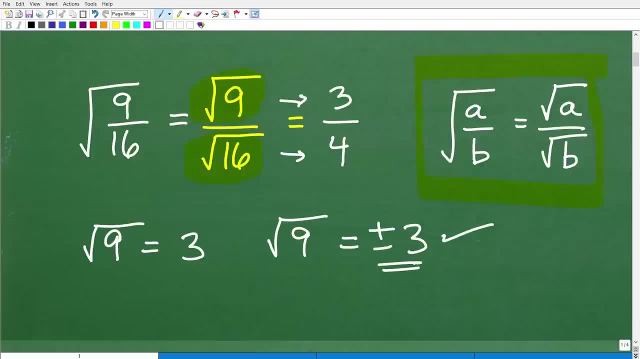 Okay, the square root of 9 is equal to plus or minus 3.. And this is really going to be applicable when you're solving equations, finding roots, etc. When you're doing a problem like this, you just go ahead and write that principal square root, which is just going to be the positive version of this answer. 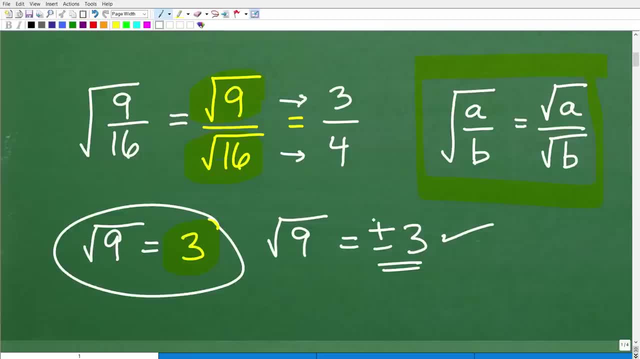 So don't feel compelled to have to write both positive and negative in your answers, okay. So this is from my experience. But again, you want to check with your teacher when you're doing these problems. But typically you're just going to be asked to find the principal square root, which is just the positive version. 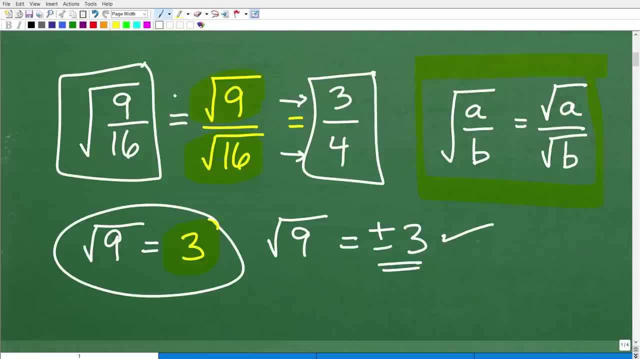 Okay, so the square root of 9 over 16, or 9 sixteenths, is equal to 3 over 4.. And the main principal, here again that we're using the principal of square roots, is the square root of a fraction: a over b is equal to the square root of a over the square root of b. 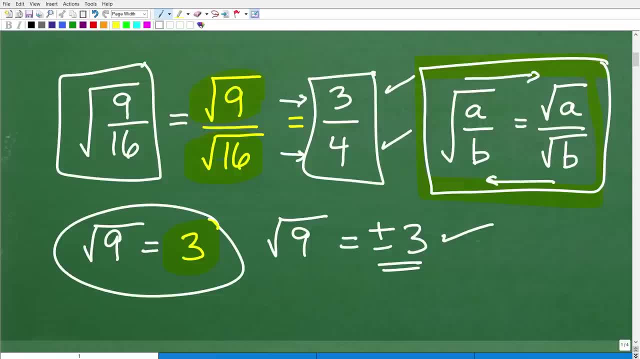 So you can either go this direction or this direction, right. So this is a principal or a property of square roots that you need to commit to. It's your long-term memory. But if you knew that, that's excellent. And now let's move on to our next problem. 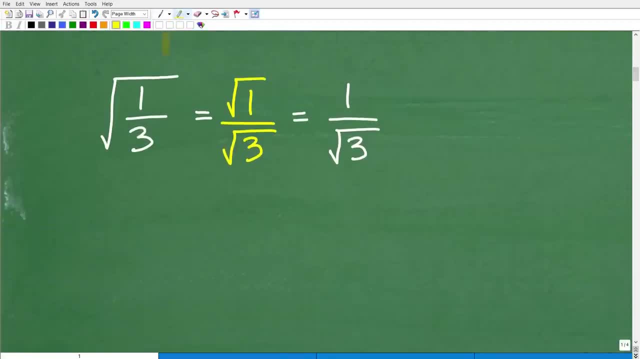 Okay. so here we have the square root of 1 third. So, knowing this principal, I'm going to say, okay, I'll just take the square root of the numerator, that's, the square root of 1, over the square root of 3.. 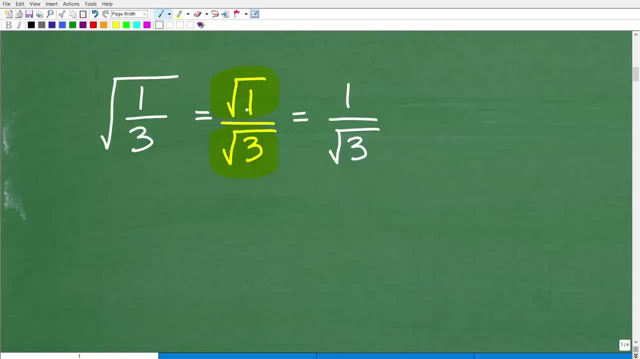 Okay, I'm just applying this property I just showed you right now, And the square root of 1 is 1, and then the square root of 3 is just the square root of 3.. Okay, so Now how many of you think this is a good answer? 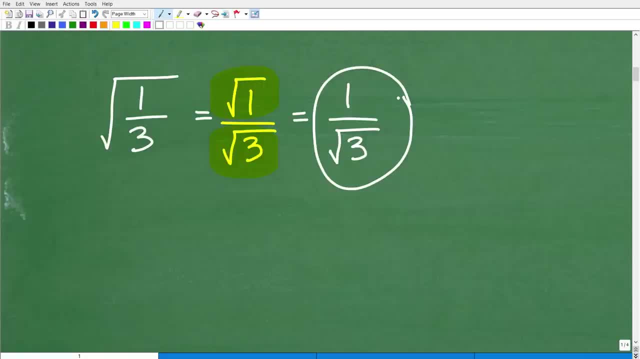 Okay, are you saying, or would you turn this answer in for credit on a quiz or test? So if you would, you'd be like, oh yeah, that looks pretty good to me. Well, unfortunately, I have to give you a sad face because this is not correct. 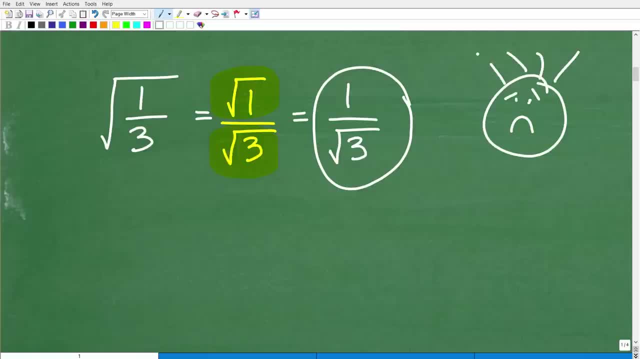 So, as some of you are saying, what are you talking about? It's not correct. You're just showing me what to do here. Well, we have a problem. okay, This is correct up to this point, but we're not done okay. 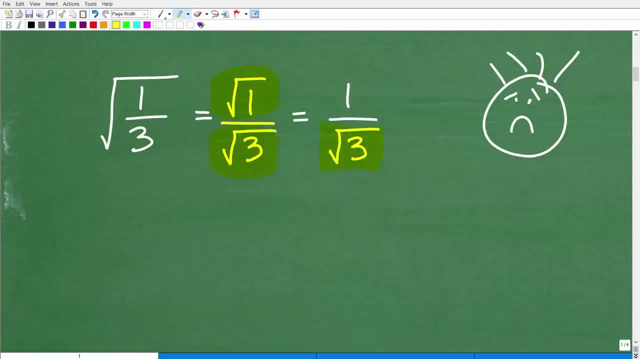 We have 1 over the square root of 3.. The square root of 3, right here is something we would classify as an irrational number. okay, An irrational number. Now, on a number line we have different numbers. So here's 0,, here's 1, here's 2, here's negative 1, here's negative 2.. 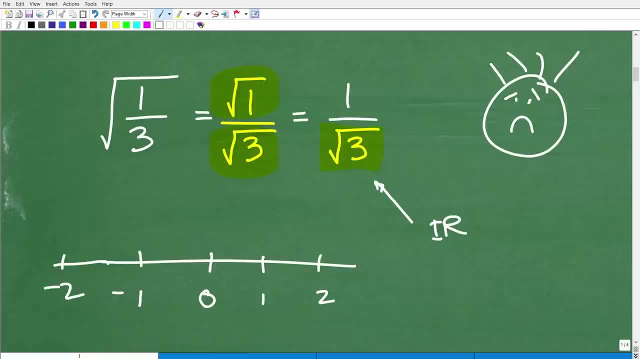 So we have all sorts of numbers on the number line, okay. So we have natural numbers, whole numbers, integers, Irrational numbers and then something called irrational numbers. So irrational numbers are numbers like the square root of 3 or the square root of 7.. 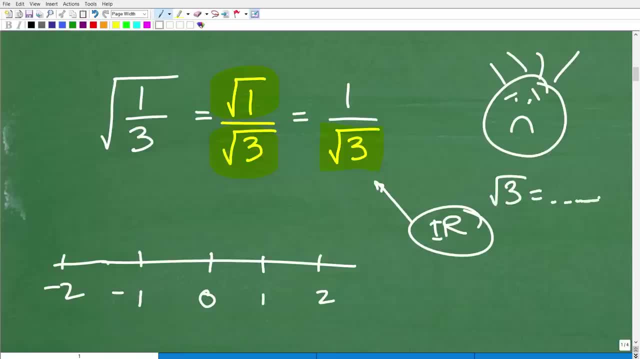 So if you go into your calculator and you go to the square root of 3, you're going to get a decimal. okay, You're going to start getting some sort of decimal answer And your calculator is going to continue on with this decimal. 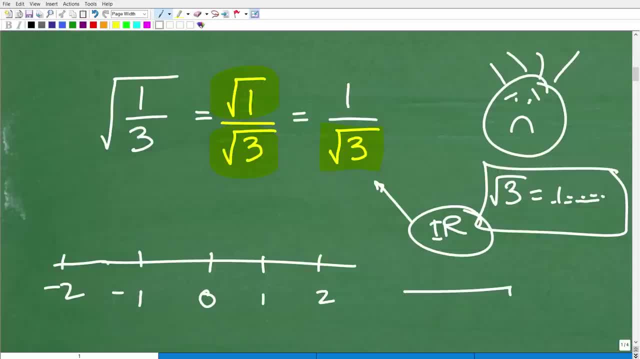 This answer, okay, in terms of a decimal, never ends. This decimal goes on forever and ever and ever. It's what we call non-terminal, It's what we call non-terminating and non-repeating. okay, So here we're trying to divide 1 by a decimal that never ends. 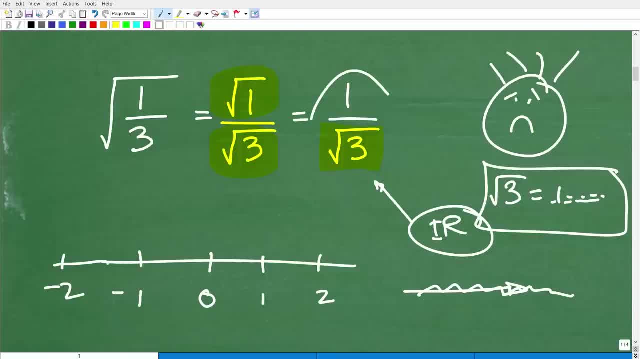 It never stops, It never repeats itself. So in mathematics we do not like that. We do not like to divide a number or have in the denominator an irrational number. okay, So let's just make sure we're super clear about this, because a lot of you might get confused. 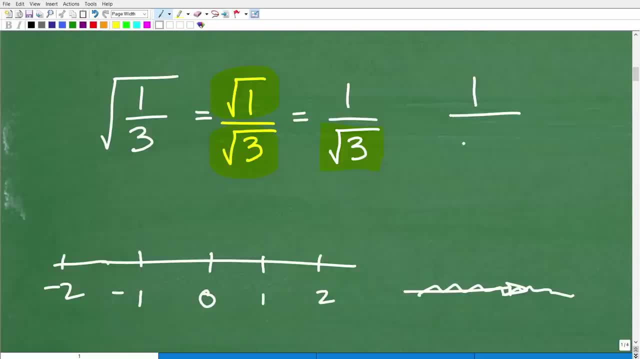 Let's take a look at this. What if I had 1 over the square root? What if I had 1 over the square root of 9?? So you might be saying, well, there's a square root, Isn't this an irrational number? 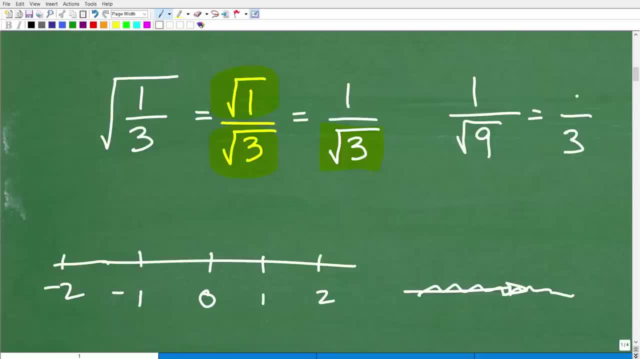 No, because 9, we could take the square root of 9.. That is simply 3.. So that's one-third. no problems, okay. However, the square root of 3 is an irrational number. So this is a problem, okay, the way it's written right now. 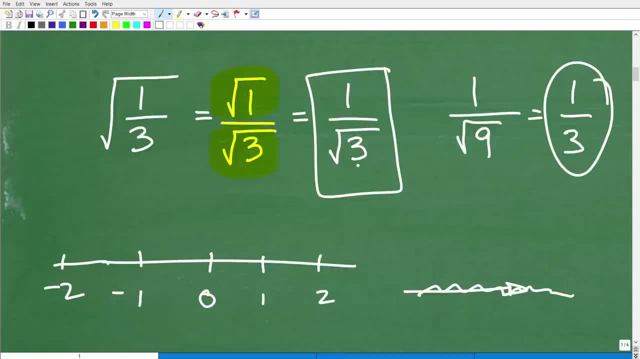 So we're going to have to do something about this, And luckily, we have a procedure that we're going to do, And that's called rationality. We're going to rationalize the denominator. okay, We're going to rationalize the denominator. 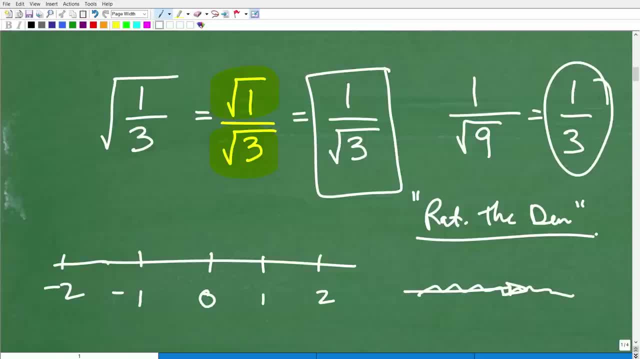 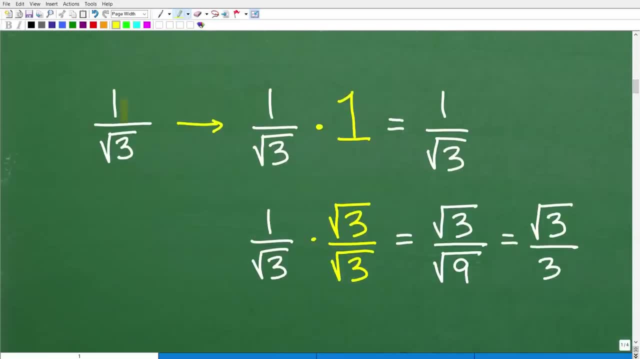 That's the term, And, of course, I'm kind of just using some shorthand here. So what does that look like? Well, I'm going to show you this right now. Okay, so here we could see: our answer is 1 over the square root of 3, but it's incomplete. 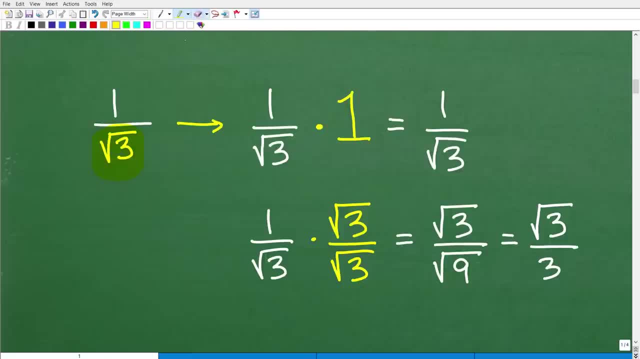 because we have this irrational number down there. So what we're going to do is we're going to kind of use a little trick. So we're going to take this 1 over square root of 3. This is our number And we're going to multiply it by 1, okay. 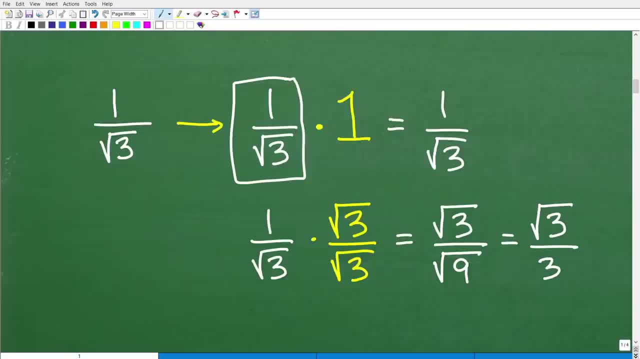 So if you take a number and you multiply it by 1, what's the answer? Well, it's just the number right? So if I take 1 over square root of 3 and multiply it by 1, it just goes back to 1 over the square. 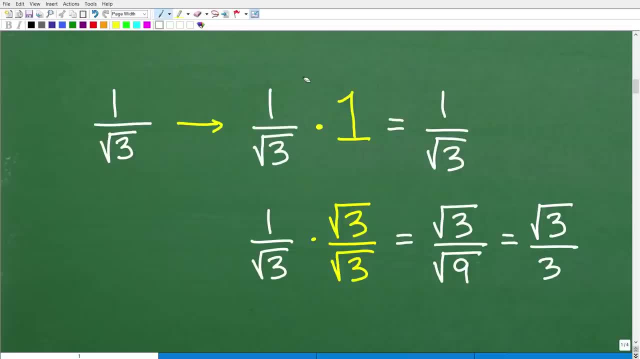 root of 3, okay, So that's pretty straightforward. But this 1 that I'm going to multiply this 1 over square root of 3 by is going to be a fancy 1, okay, I'm just not going to use the number 1.. 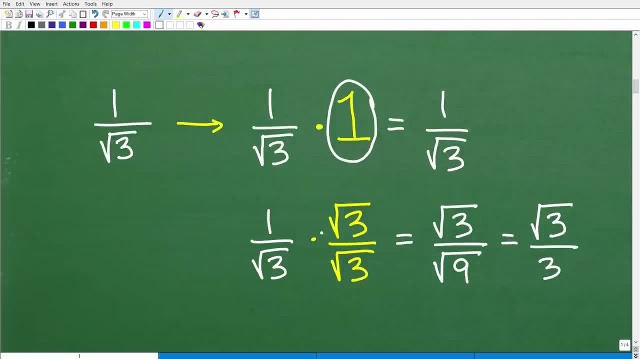 I'm going to use a number, I'm going to use another version of 1. And that is going to be the square root of 3 over the square root of 3.. So let me ask you: any number divided by itself is equal to what? 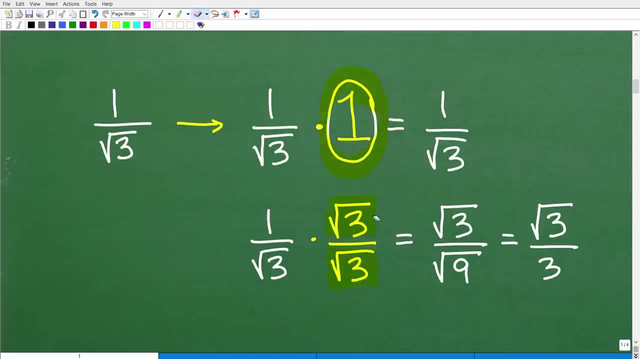 Well, hopefully, you said 1, right, So that is the case. So any number divided by itself is 1.. So what we're going to try to do here is we're going to rewrite this 1 over square root of 3, so we don't have a square root of 3 in the denominator. 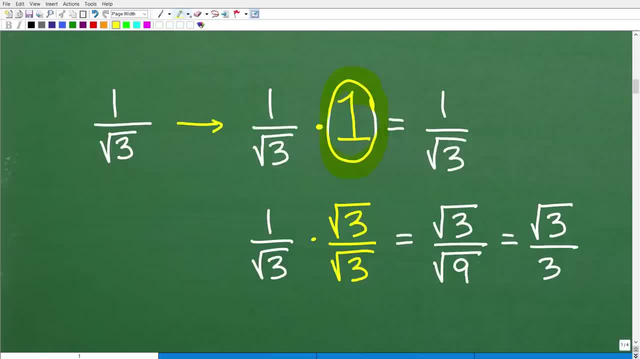 And the way we're going to do that is called rationalizing. So the procedure is this: Whatever the radical you're dealing with here, it's square root of 3, we're going to multiply by a fraction square root of 3 over square root of 3, okay. 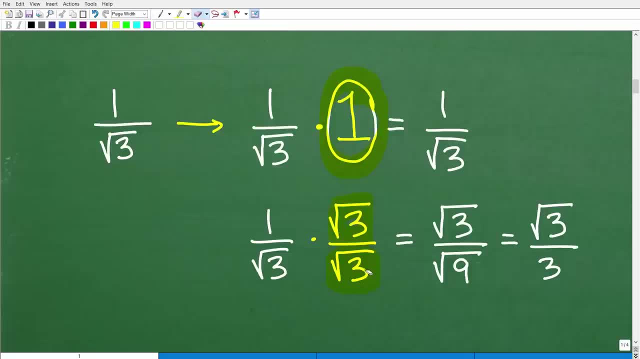 We're not breaking this thing, because the square root of 3 divided by the square root of 3, again is 1,. okay, So you don't have to concern yourself by saying, oh, we're changing the problem. Well, no, because this whole thing right here is in fact equivalent to 1, but we are going. 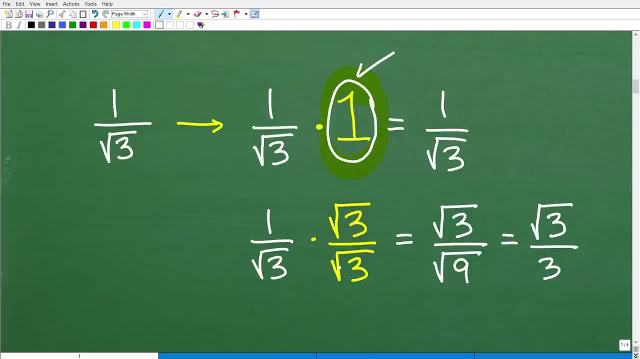 to make it look different. Okay, And now let's go ahead and actually do this math. So now we're going to take 1 over square root of 3, and we're going to multiply it by the square root of 3 over the square root of 3.. 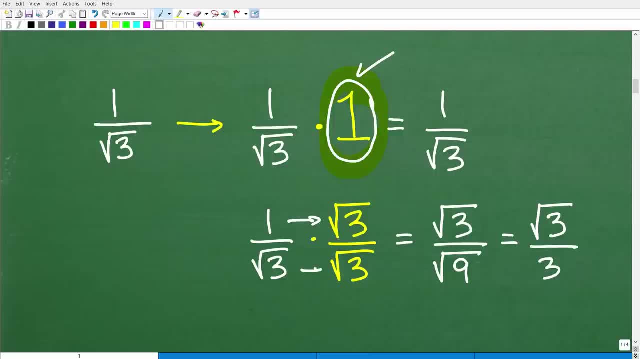 This is called rationalizing the denominator. So here we have 1 times the square root of 3.. That is the square root of 3.. And then the square root of 3 times the square root of 3 happens to be equal to the square. 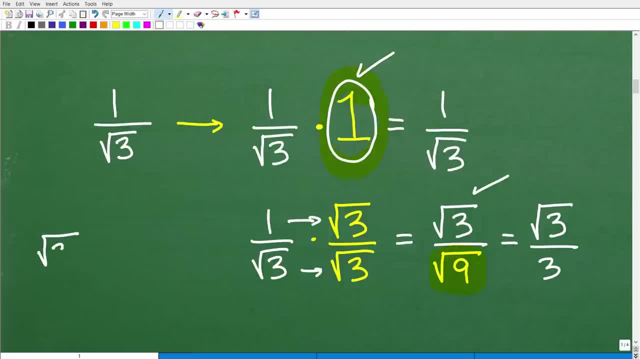 root of 9.. So when you're multiplying square roots, like the square root of 3 times the square root of 3, that's equal to the square root of 3 divided by the square root of 9.. Okay, So that's 8 times 3, just in case you don't remember that. or the square root of 9.. 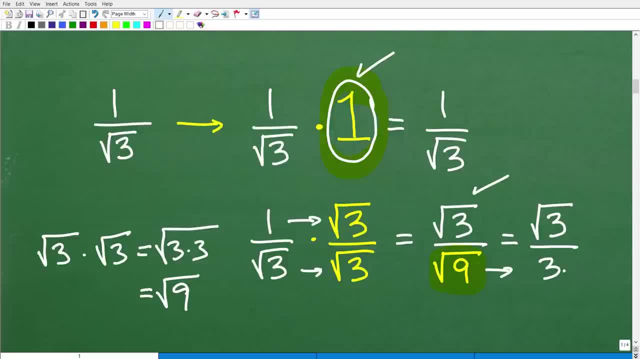 So now we have the square root of 3 over the square root of 9.. Of course, the square root of 9 is equal to 3.. Now look at that. Okay, We have a nice, lovely whole number in our denominator, and that's perfectly fine. 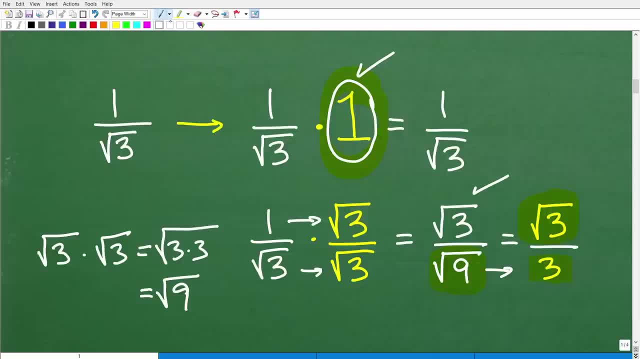 Okay, So now we have the square root of 3 over 3, and this, mathematically, is equivalent to 1 over the square root of 3.. But we like this much better Because it doesn't have an irrational number in the denominator. 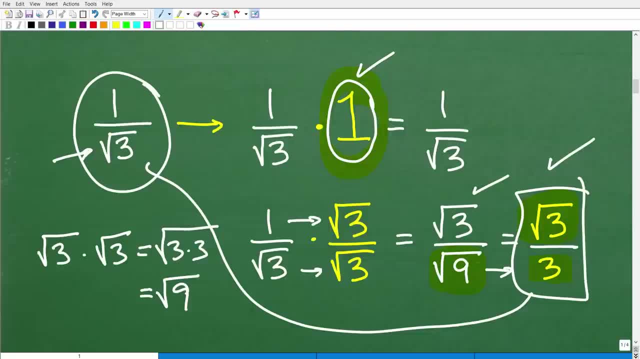 Okay. So very, very important concept: when you're working with fractions and square roots, You've got to make sure you rationalize any fraction that has an irrational number in the denominator. Okay, If you do not do that, you will get points taken off on tests and quizzes. 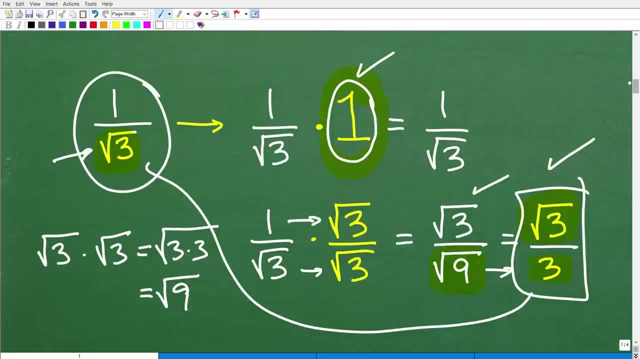 Okay. So let's bring um, or let's go ahead and go to our last problem, Or this brings us to our last problem. So here we have 4 over 1 plus the square root of 8. Okay, 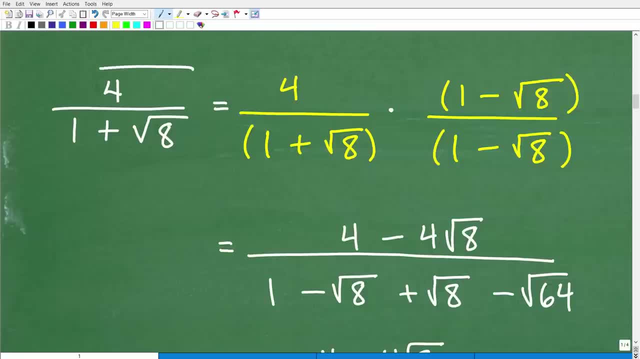 So this is the expression. So some of you might be thinking: alright, uh, Mr YouTube Math Man, are you thinking that we're going to have a problem with this square root of 8?? Uh, because this is an irrational number in the denominator. 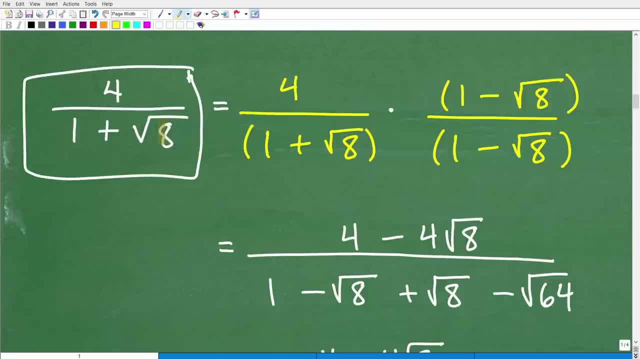 Do we need to do something about that? Well, if that's what you're thinking, you would be absolutely correct. This is a problem, Okay, So we're going to have to rationalize it. We're going to have to do something about it. 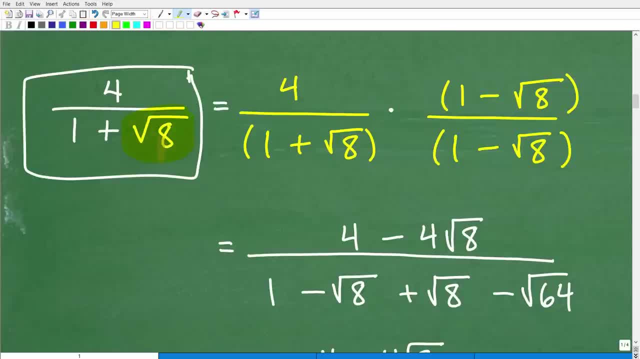 Okay, So we're going to have to rationalize it. We're going to have to rationalize it. Okay, So we're going to have to rationalize it. This is an irrational number in the denominator. Do we need to do something about that? 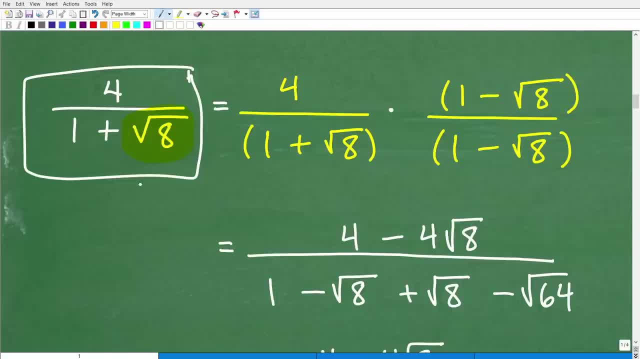 Well, if that's what you're thinking, you would be absolutely correct. This is a problem, Okay, So we're gonna have to rationalize this, but this is different than the previous problem that we just did. Okay, In the previous problem, we had 1 over the square root of 3 and we only had one. uh, you, 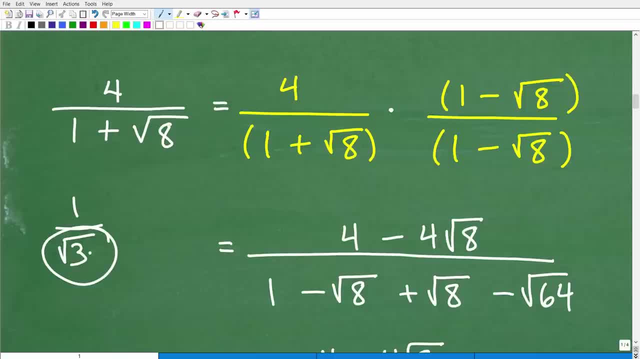 know square root all by itself, so it was easy to rationalize. How do we rationalize right here? We have 1 plus 6.. the square root of 8. well, we're going to have to multiply this entire fraction by something called. 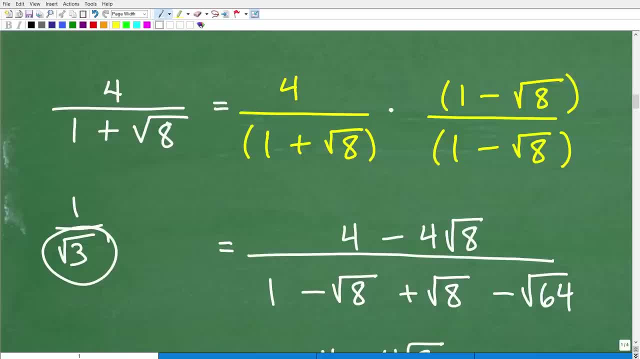 the conjugate. okay, the conjugate and the way that works is this. so let's take a look at our denominator. we have 1 plus the square root of 8. the conjugate is going to be the same numbers. okay, 1 and the square root of 8, but the different sign. so if this is plus, this is minus, so this is. 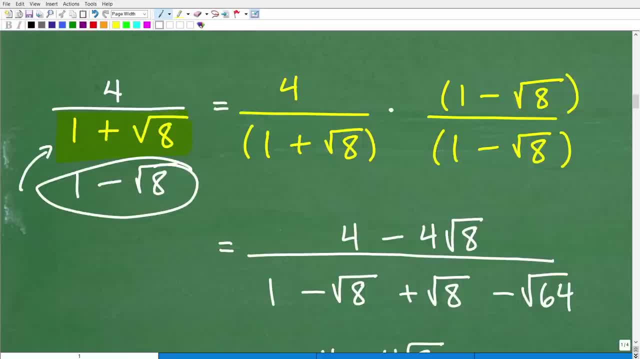 the conjugate of this. okay. so let's do another example here. what if I had 2 minus the square root of 5? what would be the conjugate? let's say that was in our denominator. the conjugate would be 2 plus the square root of 5. so it's basically the same thing. you just change the signs, okay. 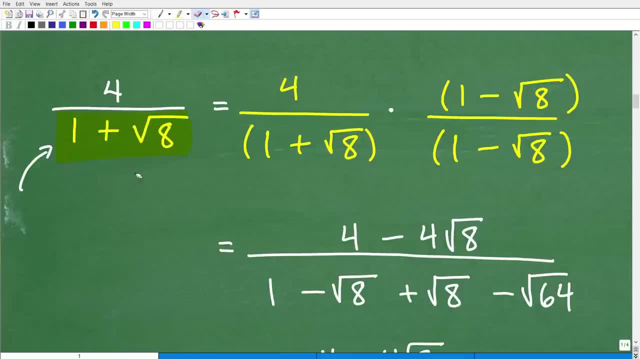 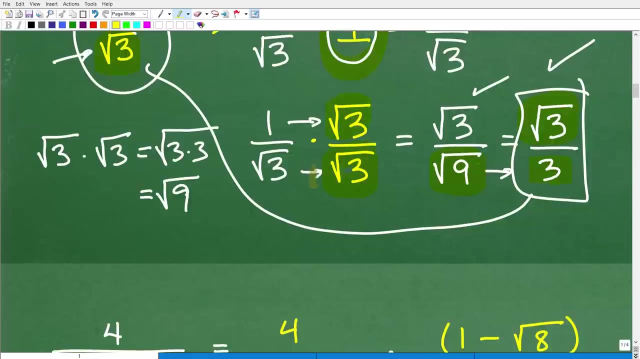 so now what we're going to do is we're going to multiply both the numerator and denominator. that's basically the same thing that we did last time. let's just go back here real quick. we multiply both the numerator- I'm sorry, the numerator- and the denominator by the square root of 3. over here we're going to multiply the numerator and. 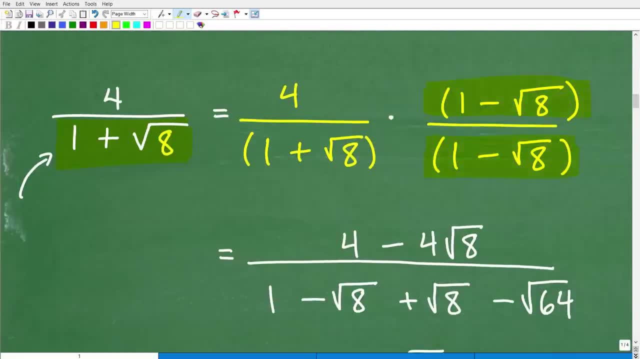 denominator by the conjugate, which in this case is going to be 1 minus the square root of 8. okay, so you're going to have to be pretty good at dealing with multiplications of binomials. in other words, can you multiply, let's say, 2x plus 3 times? 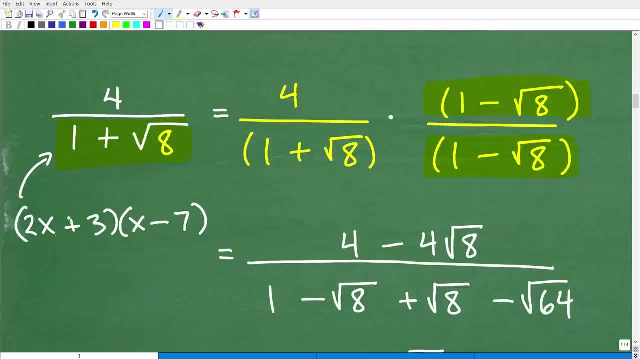 x minus 7. okay, how would I multiply these two binomials? hopefully you remember the foil method: f o, i, l. okay, if you don't remember that method, I teach all this stuff in all my algebra courses. I have tons of videos on this on my youtube channel as well. but basically you're going to 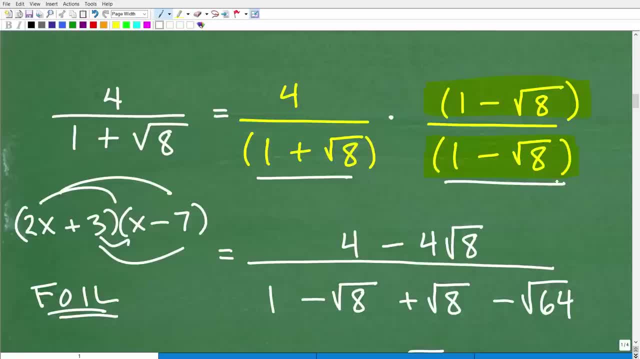 you're going to have to multiply these two expressions- 1 plus the square root of 8 times 1 minus the square root of 8- using the same technique, as a FOIL technique. In other words, you're going to have to look at these as two binomials. Okay, so the FOIL technique stands. 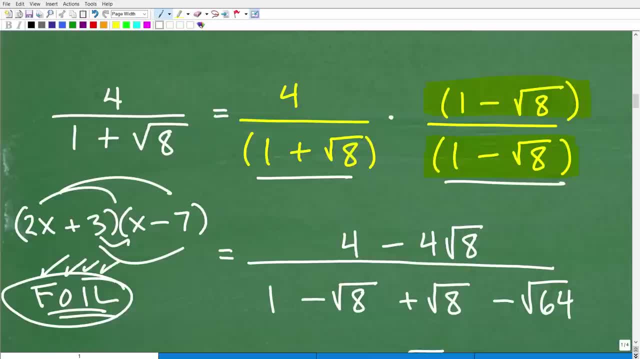 for first outer inner last. If you don't know what I'm doing here, you definitely need to do some review, as you're not going to be able to do this problem without understanding the FOIL technique. Okay, so let's go ahead and get into this, And we'll start off first by multiplying. 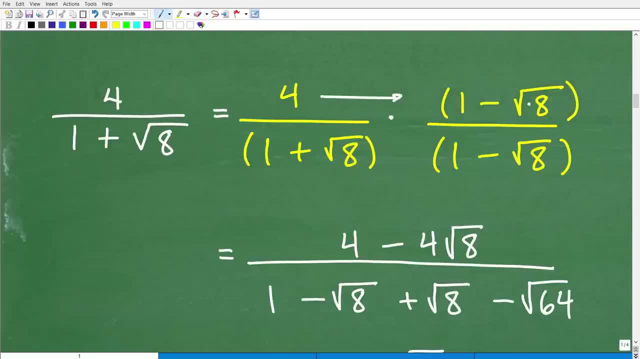 4 times 1 minus the square root of 8.. So what does that look like? Well, we can kind of scoot this 4 right here. So this is 4 times 1 minus the square root of 8.. So when I use the distributive, 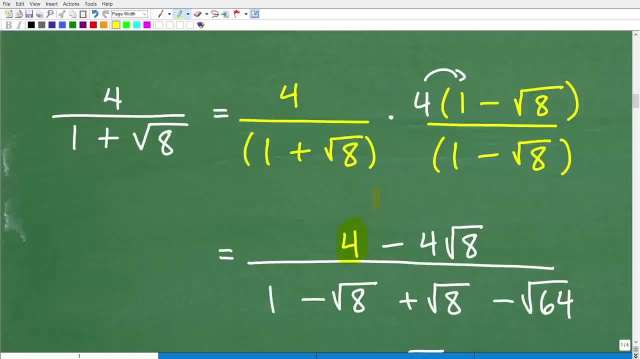 property: 4 times 1 is 4.. And then 4 times this, square root of 8 is going to be 4 square root of 8.. So there is our numerator. Okay, All right, so now we have to go ahead and deal with this. 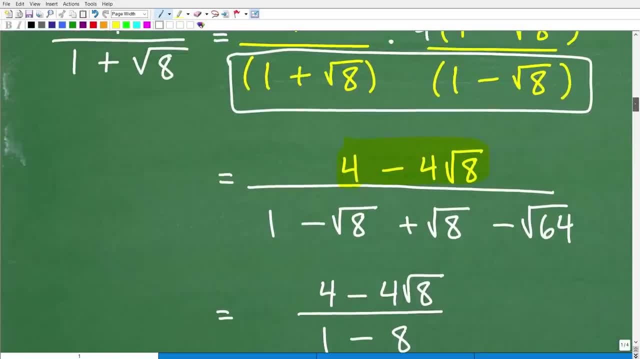 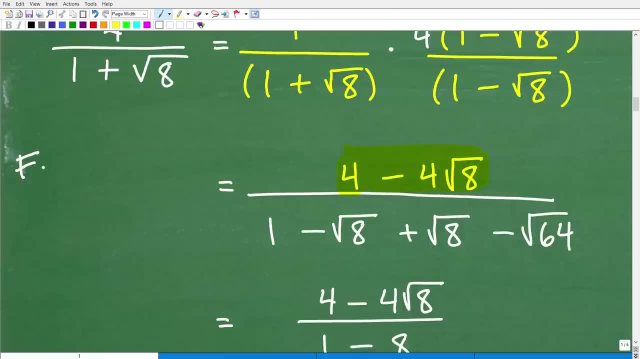 denominator, And let me go ahead and walk you through this right now. Give myself some room, All right, so let's just focus our attention here And again, we'll use the FOIL technique. first, outer, inner, last. So the first is going to be: these are the first terms of each of these. 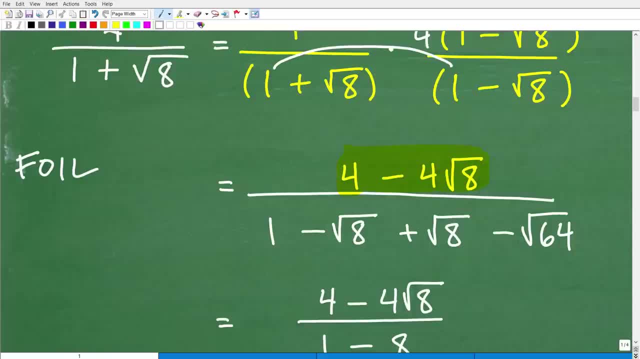 respective binomials. So 1 times 1 is 1.. Okay, So outer is going to be 1 times negative 8, which of course is negative 8.. So then I'm writing this out right there: Inner is going to be the square root of 8 times a positive 1.. So that is going to be a positive. 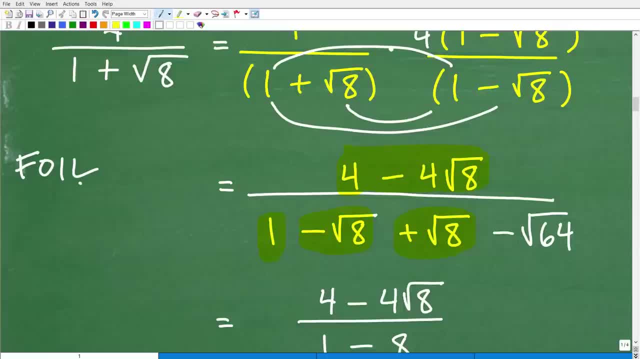 square root of 8.. And then the last terms is going to be square root of 8 times another square root of 8, which is going to be a negative square root of 64. Because this is positive, that's times positive, times a negative, So we have a negative square root of 64.. Okay, So hopefully you're with. 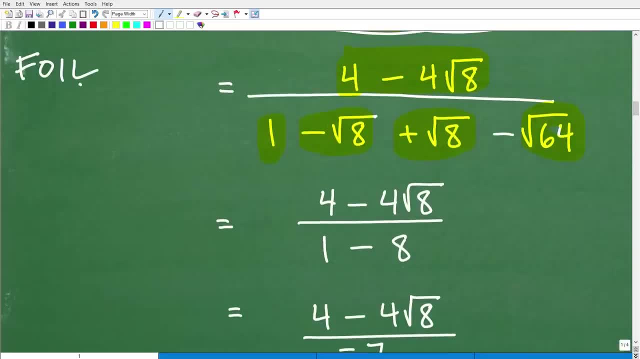 me on this. Now let's go ahead and clean up This denominator here. So what happens? Well, you can see, our square roots are going to go away right here. It's this negative square root of 8 plus square root of 8.. These are going to cross. 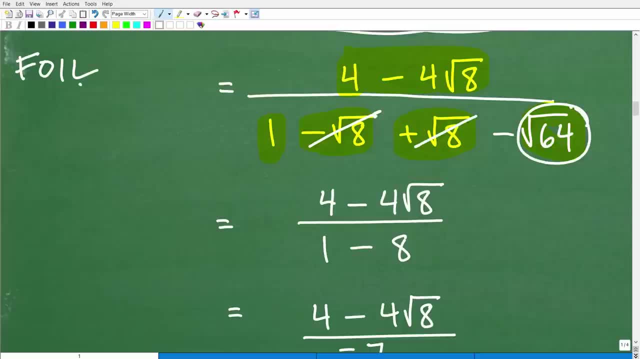 cancel Those, go away, And then the square root of 64 is 8.. Okay, Again, we're talking about the principal square root, So we're left with 1 minus 8.. Okay, This is again the result of using the. 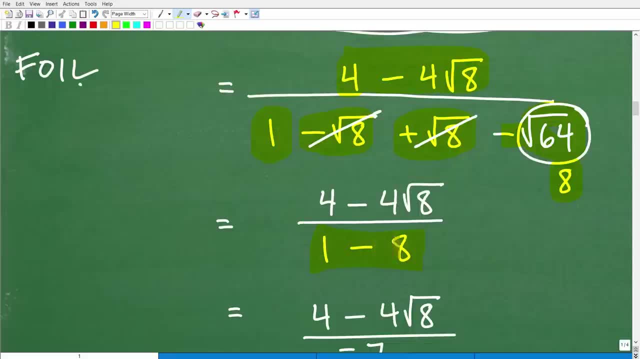 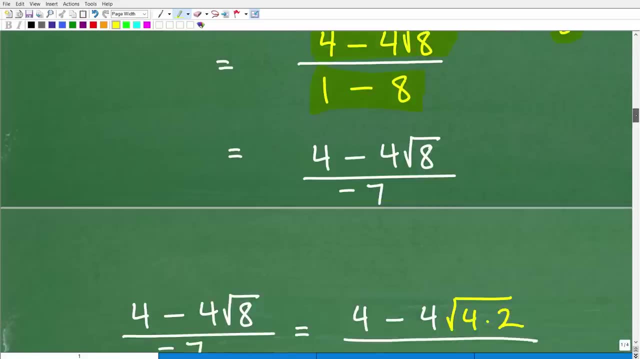 conjugate. to rationalize. Now, notice, we don't have any square roots now in the denominator, And then we have our 4 minus 4 square root of 8 in our numerator. So let's go ahead and continue forward. Now. if you're thinking to yourself: this is a lot of work, Well, you would be correct. 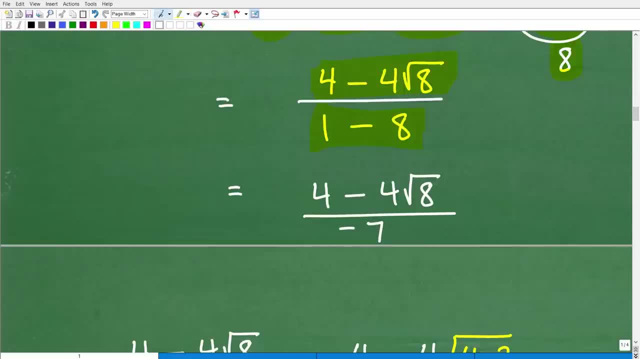 Again. you know, to deal with these expressions in algebra does require a lot of concentration and skills, but we're still not done. All right. So we have 1 minus 8, which of course is negative 7, right here. So 4 minus 4, square root of 8 over negative 7.. Are we done? No, we are not. 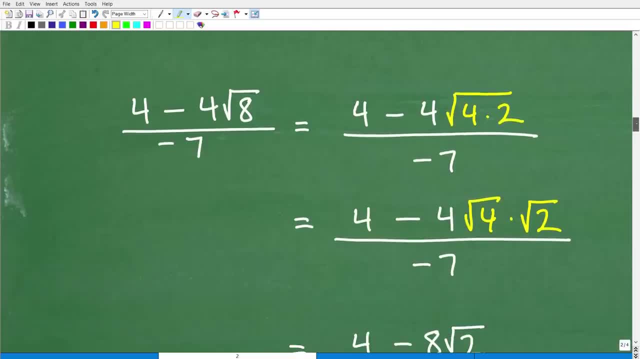 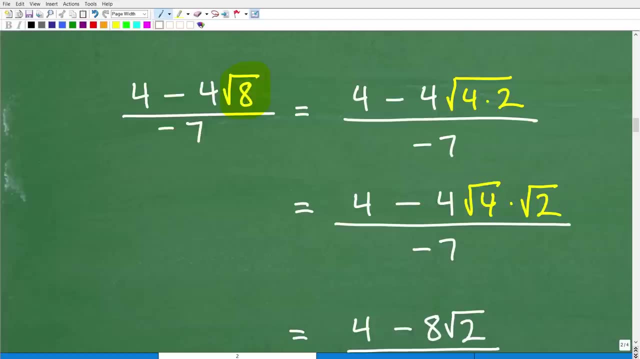 done. So you're like, oh, my goodness, this is like the problem that never quits. Well, we're almost there. Okay, What we need to do is simplify this square root of 8.. Okay, So let's go ahead and. 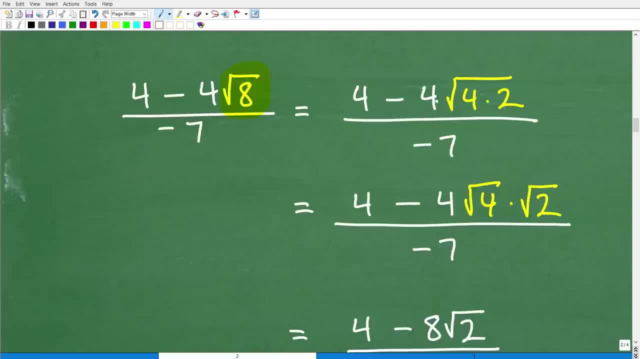 show you how to deal with this. So the square root of 8 is the same thing as a square root of 4 times 2.. Okay, So this is the way I can write the square root of 8. And I can break up this big radical. 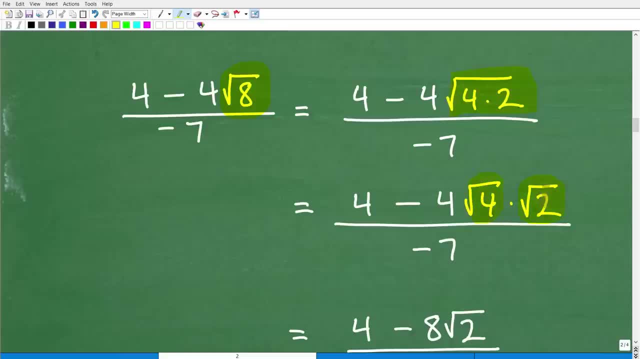 here the square root of 4 times 2, as a square root of 4 times a square root of 2.. So you want any perfect square. So the square root of 4 is what That's going to be: 2.. So this is going to. 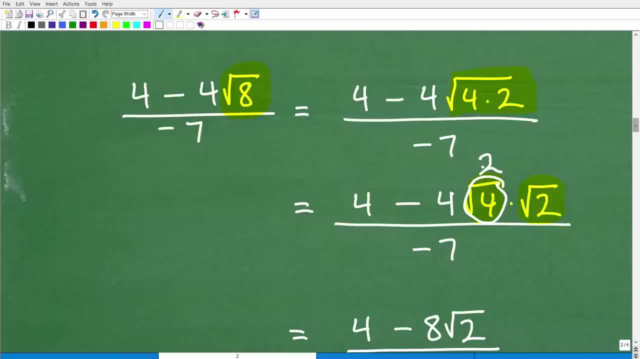 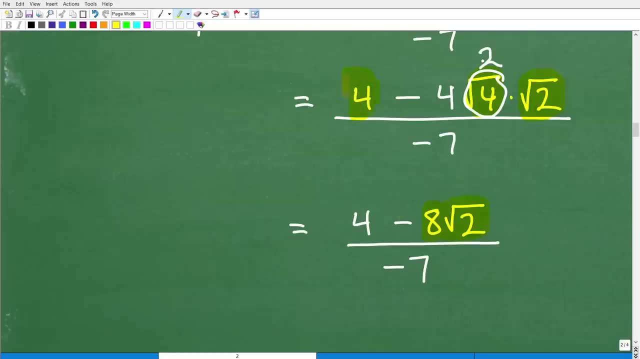 be 4 times 2, which, of course, is 8.. And that's exactly what we want to write. So this is going to be 8 times the square root of 2.. That's what's remaining there, And, of course, we have 4, right. 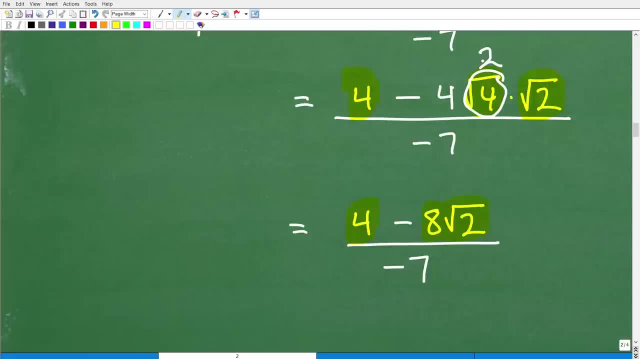 there as the part of our expression in the numerator over this negative 7.. And now we are done. There's nothing here that we can, no greatest common factor that we can cross cancel. So we are finally, finally done, Okay. So yes, there is a lot involved when you're dealing with 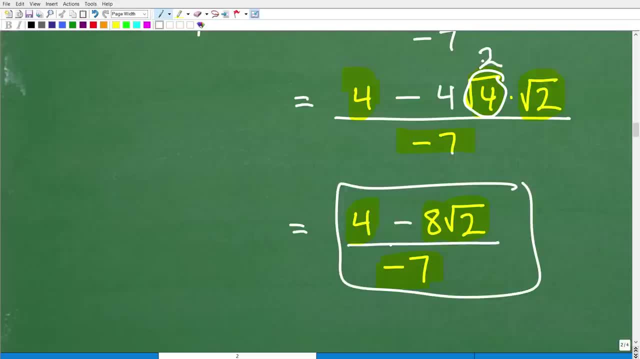 square roots and fractions. I'm trying to pick three problems that are going to kind of, you know, represent the type of things you're going to see in algebra. But if you got all three of these right, I must go ahead and give you a nice, lovely, happy face. an A plus plus a 130%, and 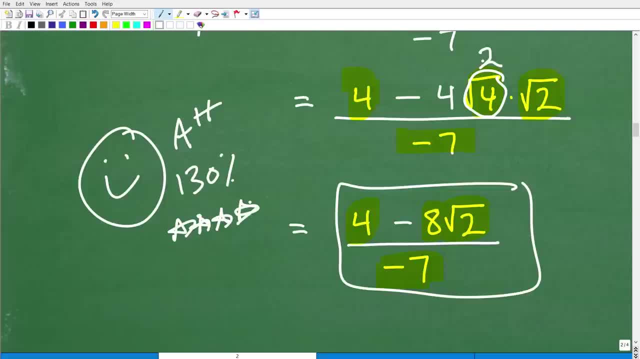 multiple stars for being such an awesome algebra student. Matter of fact, if you turn in this work and you're in my class, I might just tell you: just you know, take the rest of the year off. I'll just send you your report card and your awesome grades. But listen, in all seriousness, this is. 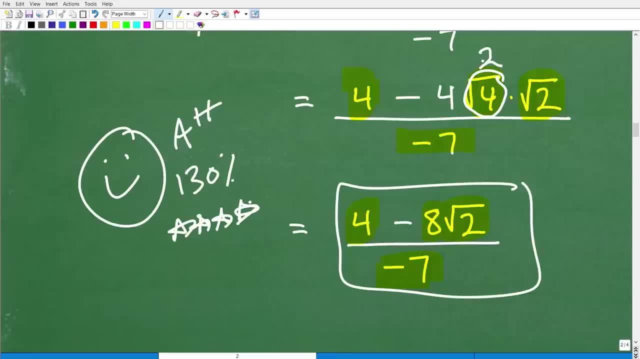 very, very good If you're able to understand this. Now, if you were like: wow, you know, I didn't know. you know, this is really hard, You know I didn't get this. Well, you need to get.